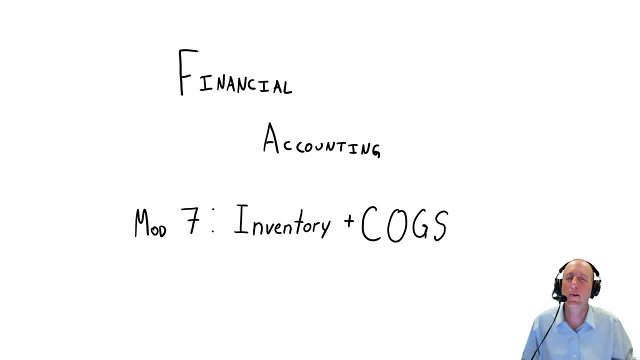 maybe you're coming at this from your own textbook. we're going to be talking about FIFO, LIFO, Weighted Average Inventory Costing methods here. So inventory and cost of goods sold is the big topic. So let's jump into what this means and why it's an issue. 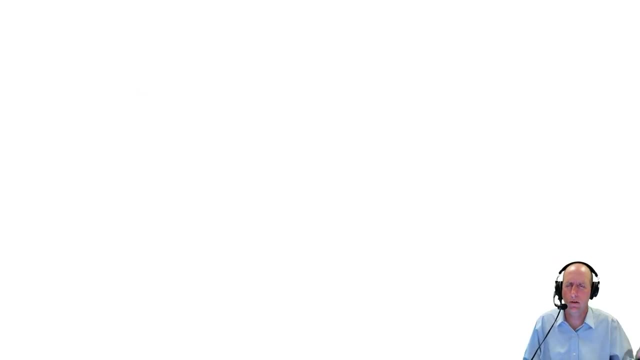 So let's say we're Walmart and we are, you know, a restaurant. We're a retailer like Walmart anyway, And we- I want to zoom in on a specific pair of socks that Walmart might sell. So you know white Hanes, you know just athletic socks. 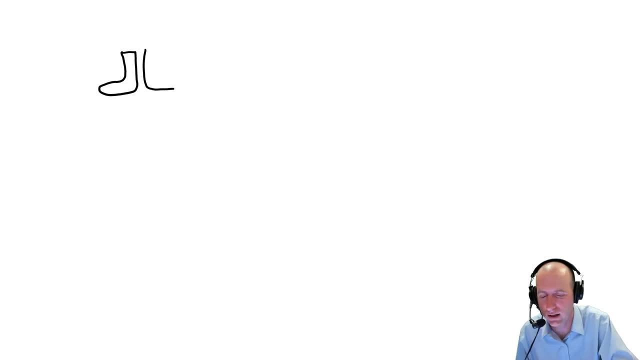 I'll draw one sock. I'm not going to draw two. I'll draw two, Why not? There's the second sock in the bear And we're Hanes and this costs us, or not? we're Hanes, we're Walmart. 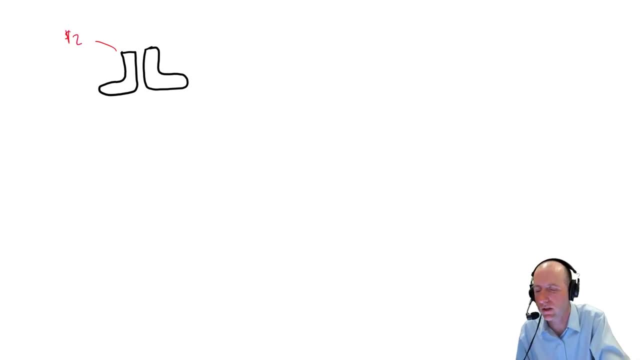 And this costs us $2.. To buy from our supplier, Hanes, and we're going to turn around and sell it to our customer for $5 for the pair of socks and we're going to make a tidy gross profit of $3. 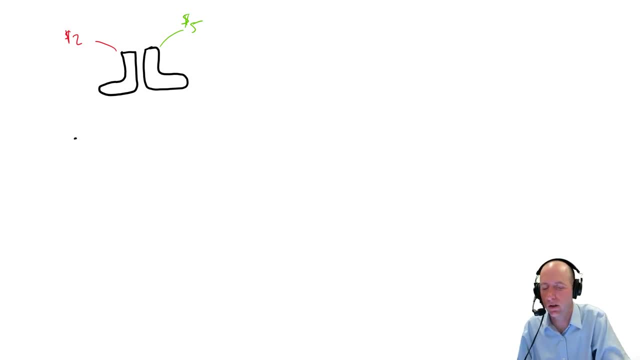 And in fact let's just do the journal entries of that simple transaction. So we buy the socks from Hanes debit inventory socks And again it would be more specific than that- We would say: you know, these are white. 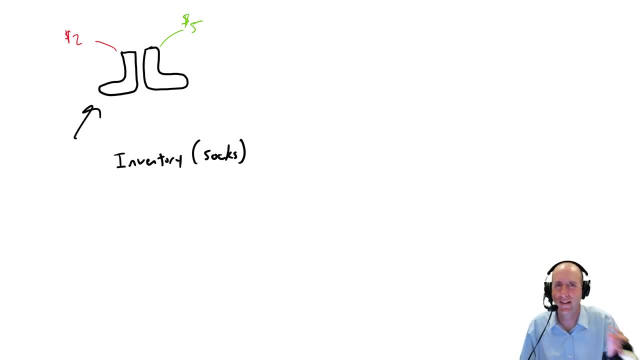 Socks this is. you know. they're large size And whatever other details we would need to distinguish. because we carry so many other pairs of white socks we would have more detail tied to it than that. But anyway, we debit inventory socks $2.. 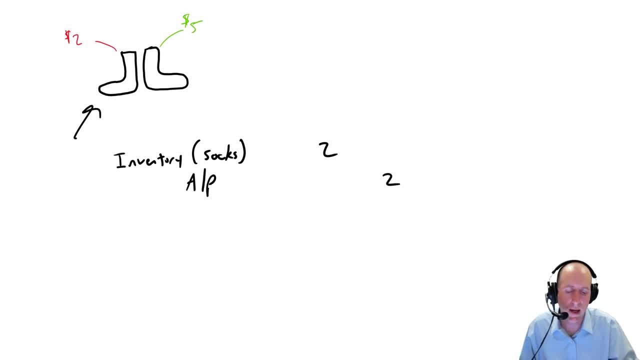 And credit accounts payable, because of course Walmart doesn't pay cash for much. And then we turn around and the next day we sell the socks. So our customer comes in and they buy the socks. So we go, okay, our customer pays us cash- $5. 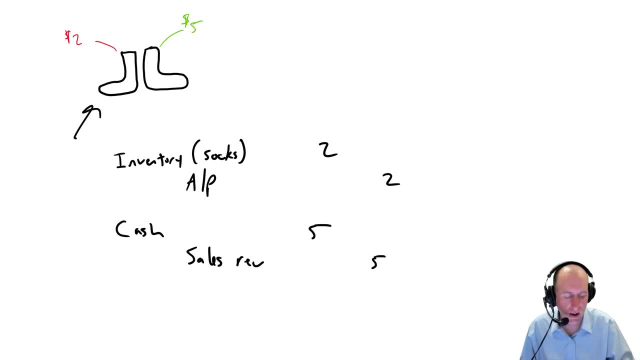 There's $6.. Sales rev of $5.. We're not worrying about any discounts or anything like this that we talked about last chapter. And of course there's two pieces to this entry. One to record: hey, there's money coming into the till the $5 amount. 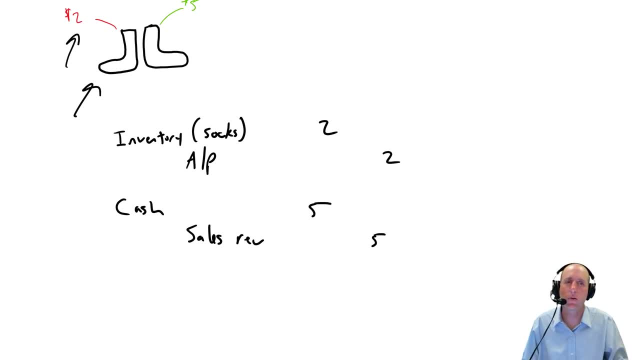 But also two $2 worth of our socks, $2 worth of our assets. walks out the door with our customers. So we credit inventory for $2. And the debit here is to cost of goods sold. So $2, and that's that special expense account. 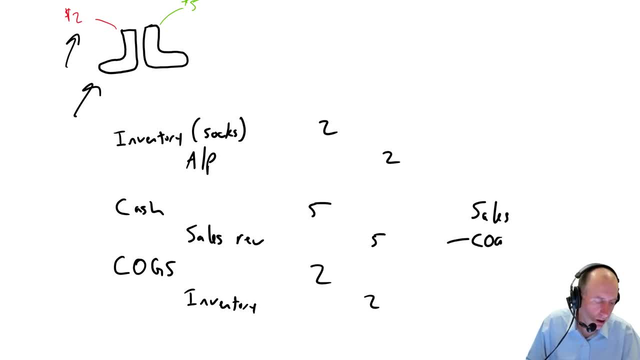 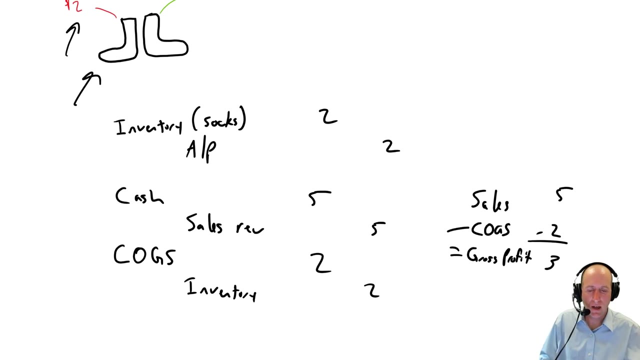 And we can see: sales minus COGS equals gross profit, also called gross margin, And our gross profit on this deal was 5 minus 2.. We made $3 in leaning out of the way of my 3.. We made $3 in the sale and that's certainly reflected in our accounting information. 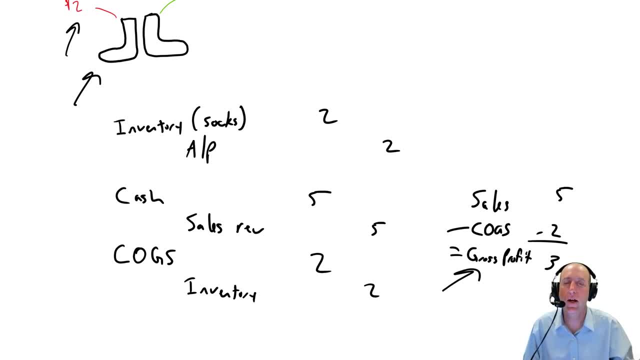 So we've done it And there is a sale. Simple example. Now here's where things get a little bit more complicated, And this is going to be the focus of our chapter. So let's assume again, Walmart buys that $2 pair of socks. 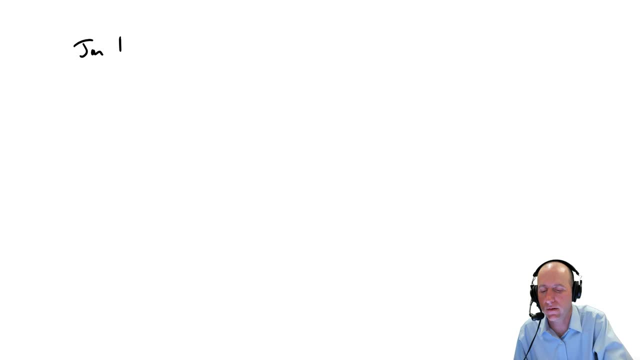 Let's say it's January 1st. So January 1, Walmart buys a pair of socks. They go debit inventory. I'm not going to say socks, but you know, you know it is socks $2,. credit AP: $2.. Let's assume that those socks do not sell. January 2nd Walmart buys another pair of socks. Now, of course Walmart wouldn't buy one pair of socks. They would buy thousands of pairs of socks at a time, But for this example, we're just going to buy one at a time. So on January 2nd they call Hanes and Hanes says: Hey, you know what? The price of socks has gone up, The price of cotton has gone up for us And therefore we've got to charge you $2.05 for that pair of socks. And Walmart eats it and they buy the socks for $2.05.. Again, Walmart probably fights. Remember this because Walmart is known as a pretty tough company, a pretty tough customer. They will be very demanding. But anyway, let's assume Walmart goes along and buys the socks for $2.05.. On January 3rd, Walmart buys another pair of socks and Hanes says: This is out of control, these cotton prices, And in fact we've got to charge you, let's say, $2.16 for our socks now. 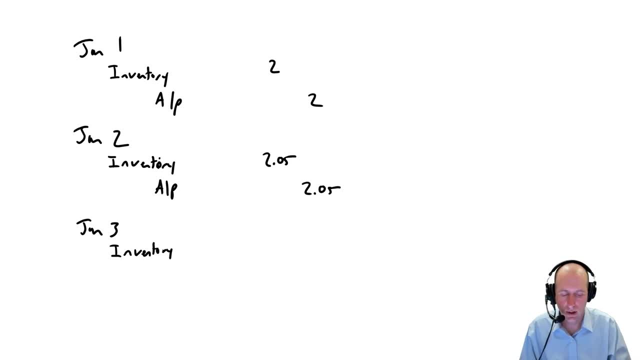 So Walmart goes Ugh. okay. Debit inventory: $2.16.. Credit AP: $2.16.. Okay, so that's all my sort of setup here. January 4th a customer comes in and they buy the socks. 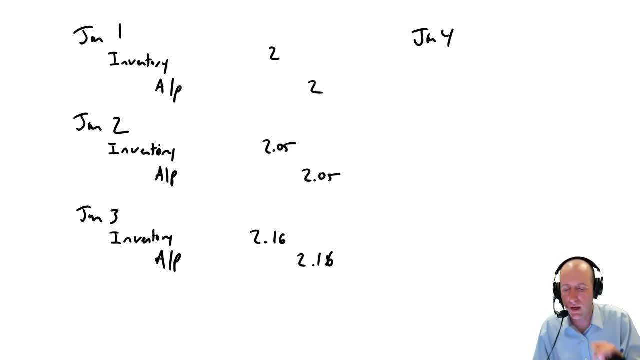 And so we have our normal sales right. And listen to be abundantly clear: these are all the same, same same skew, same type of sock. right, They come in the same, They come in the same package, They have the same everything associated with it. 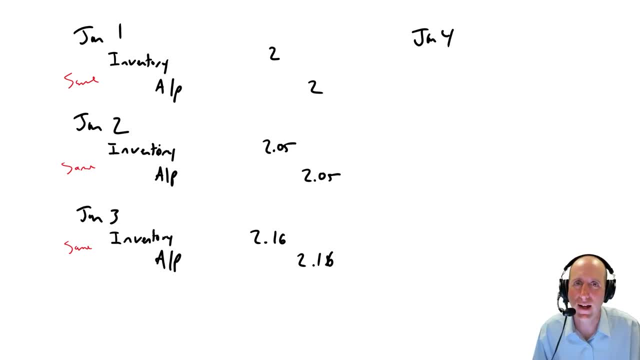 And from the customer's perspective, they all have the same price tag on them. The price is $5.. So the customer comes in and they see this pile of three socks on display- or three pairs of socks, I should say- And they buy a pair of socks. 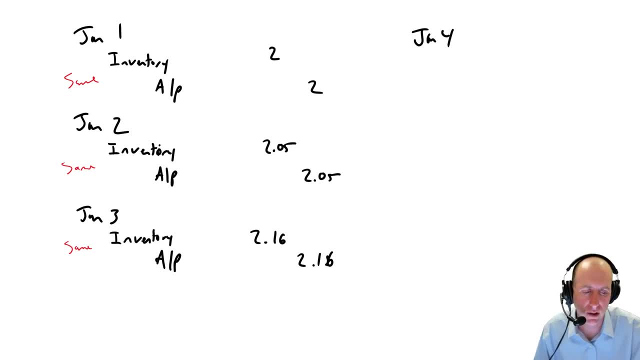 And of course they all cost the customer $5.. So Walmart receives $5 cash. They have $5 in sales revenue. The question is, what is the cost of goods sold, In other words, how much inventory walked out the door with our customer? 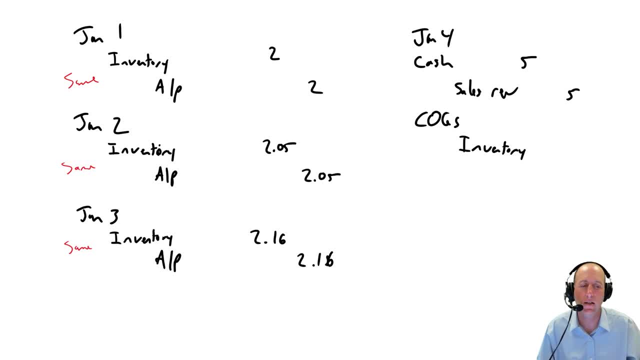 What was the value of the inventory that walked out the door with the customer? And this is the fundamental question of Module 7 here- And the answer is: it depends. And it depends on the company's accounting method. There's really four accounting methods we need to be worried about. 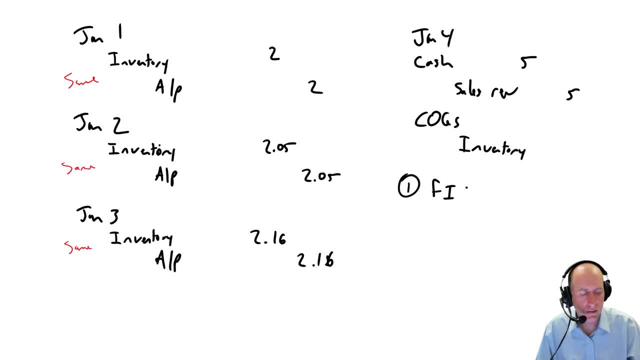 The first method is called FIFO. FIFO is short, for I should have left more space here. First In, First Out: FIFO. And what does FIFO mean? FIFO means the first one we bought, that's the first one we sold. 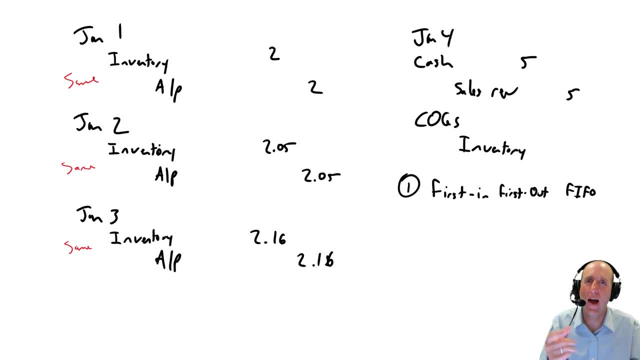 So it doesn't matter what actual pair the customer grabbed, like the top one, the bottom one or the one in the middle. First In, First Out means the oldest inventory, that's the inventory that's sold. So when I debit COGS, Credit Inventory- 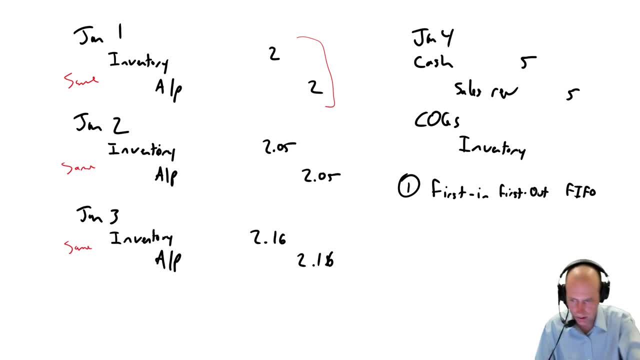 under FIFO, I'm going to debit COGS Credit Inventory for $2.. So under FIFO, COGS equals $2.. Now there's another method: Last In First Out. Now, Last In First Out is very unpopular around the world. In fact it's not a lot. It's not allowed under most accounting systems, except for there's a few notable exceptions. The main notable exception is our cousins south of the border. I'm in Canada South of the border. my American cousins are allowed to use FIFO. 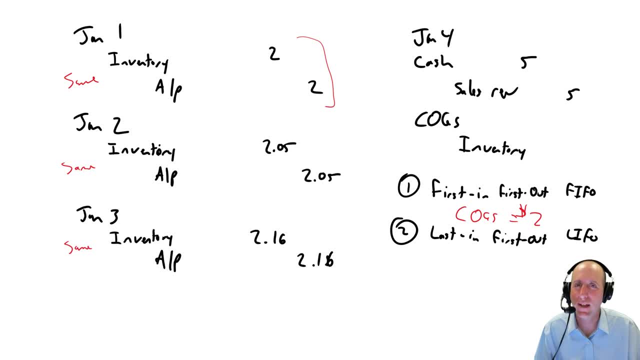 There are some specific rules around it, but I don't think it's a very good method, to be honest with you. But, that said, real companies use it, so you American students will have to know what it is. I don't require my students to know what it is. 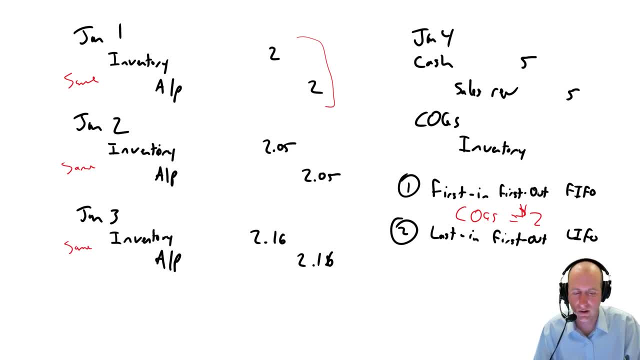 But you know, just eyeballing it, you should be able to figure out what the Last In First Out means. The last one we bought this $2.16, is going to be our COGS. Our COGS will be $2.16. 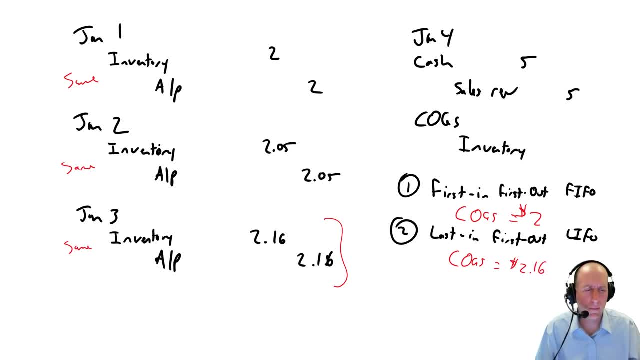 If you're curious about this, maybe you leave a comment below why I don't like LIFO. Um, maybe I'll make a video about it down the road, but it's probably a five to ten minute talk that doesn't really fit here. 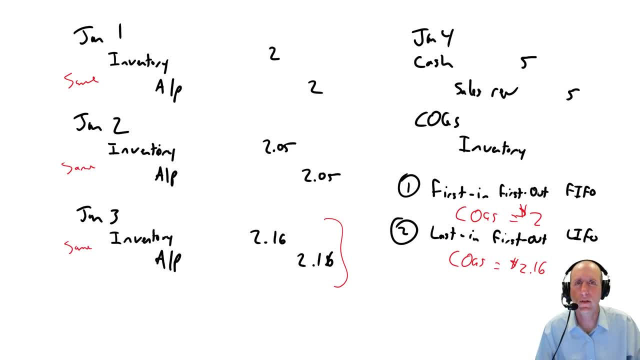 Uh, but standard setters around the world pretty much agree that LIFO is a bit uh goofy, uh anyway, Uh, okay, so that's LIFO. Uh, looking at number three, we have what's called the weighted average method. 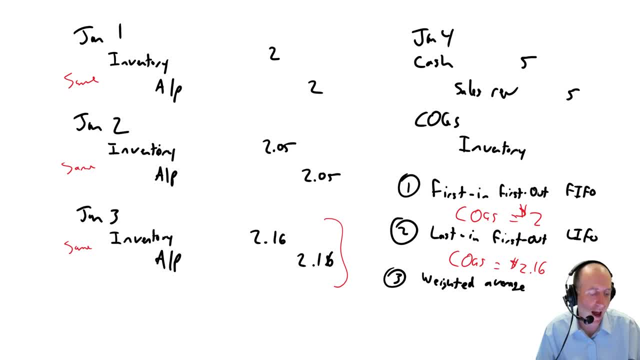 This can sometimes be called the average cost method. The the word average is going to be uh included somewhere in in uh third method And, as you might suggest, you take an average. It's not a simple average, it's a. it's called a weighted average. 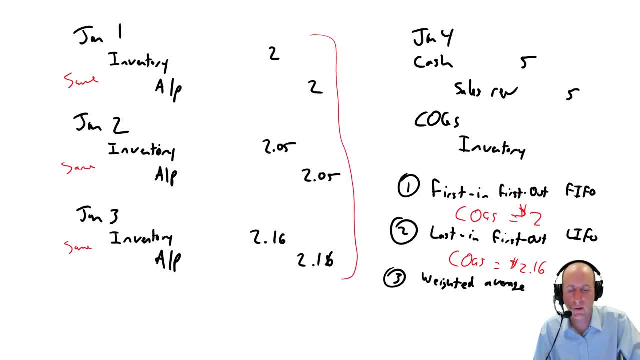 and we'll learn what that means in future videos around weighted average. But here we'll, we'll take the average of these three. So if I add two, well let me just do this in my calculator: Two, Two plus two-oh-five plus two point one-six, six-twenty-one divided by three is two-oh-seven, two dollars and seven cents. 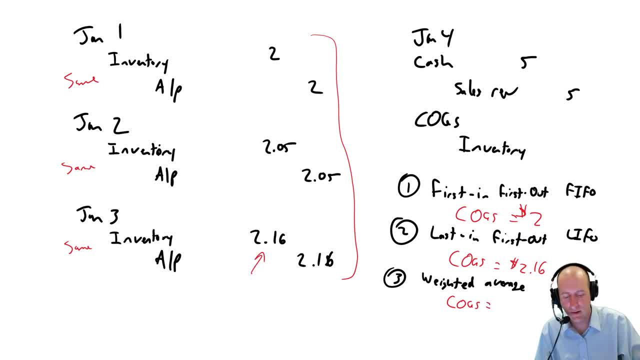 I tried to do a weighted average. The reason I chose two-sixteen here was because I thought, oh, the average is going to be an even number. Uh, I just wanted to make an even number. Of course, in real life, the weighted average doesn't have to work out to an even number. 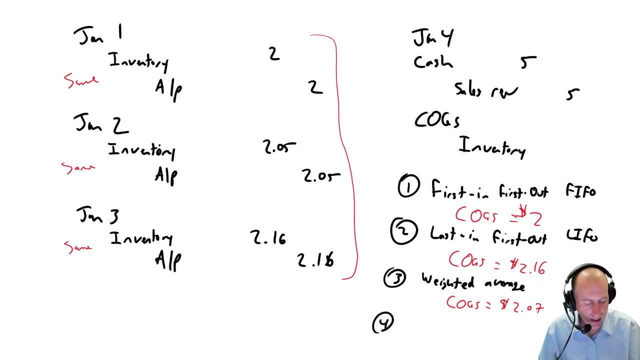 That was just my choice. The final method here is called specific unit ID, Specific unit identification, specific unit method, something like this: Um, what does specific unit ID say? Well, it says: listen if we know what pair of socks the customer took, like literally, physically. 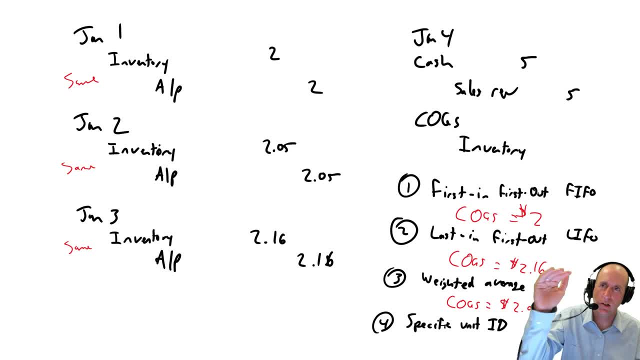 what pair of socks they took from the shelf. did they take the one that was on top did they take? did they like? when I'm buying milk, I always reach around and grab milk from the back, because that's how I roll. 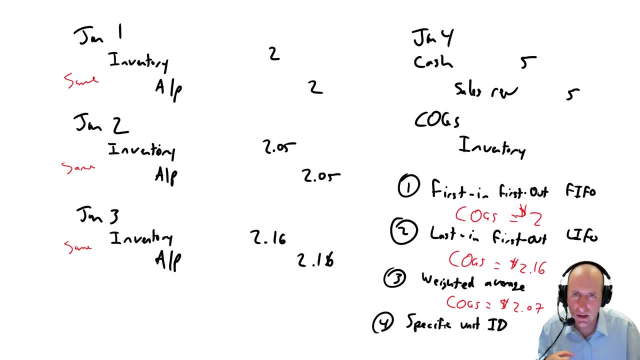 Did they grab the milk from the back, or did they grab the milk from the middle, or did they grab the milk from the front? If I'm able to keep track of that, why don't I just say the actual cost of the good that I sold right? 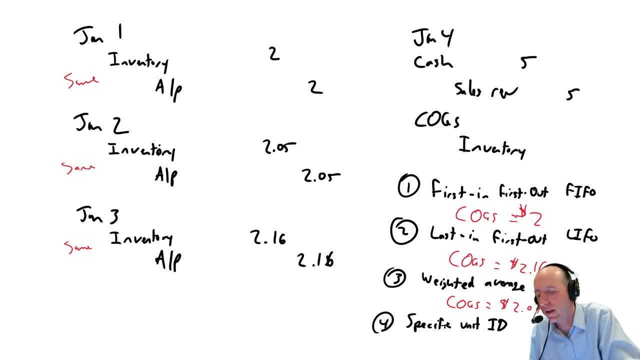 I know which one I sold. Why don't I just say: okay, well, they bought milk- number two. or they bought pair of socks- number two, therefore it's $2.05.. Or they bought pair of socks- number one, therefore it's $2.00.. 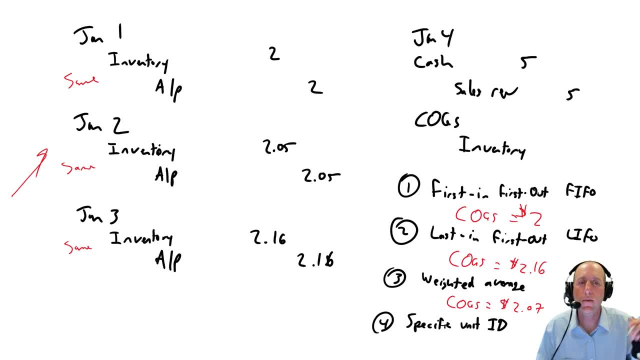 Or they bought pair of socks, number three. therefore, it's $2.16.. Whichever one they bought, that's my COGS. So in this case, COGS would, be, uh, $2.00. Or $2.05.. 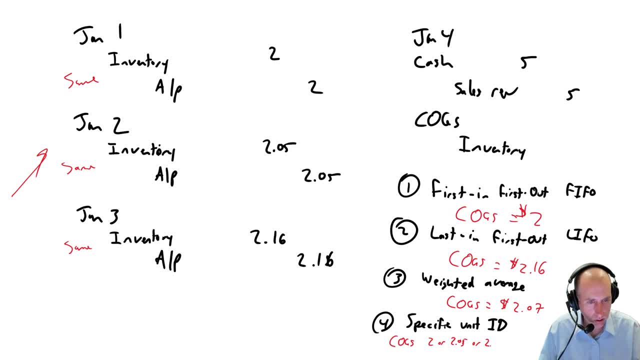 Or $2.16. Whichever one was purchased. Now, in this case we aren't sure. and if we're not sure then we can't use that method. Now, where would we be sure? Well, if I were a Toyota car dealership and I had four gray Toyota Corollas that were the same trim package, same everything. 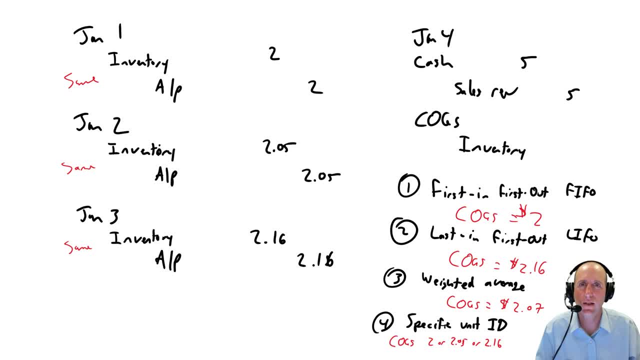 I would darn sure know which one my customer bought. It would have a vehicle ID number. I would keep track of each one separately. Or if I were an antique seller and I had, or maybe even um, let's say I was, one of these fancy painting auction houses, right? 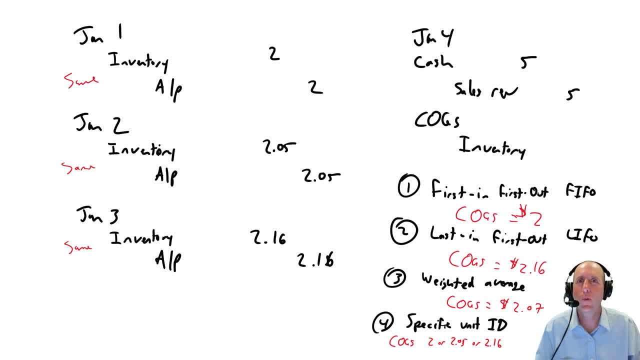 And I was selling, like paintings- Uh, I would know which was which- I wouldn't say, oh well, it's the average cost of my Picassos and I'll just average that out. No, I would keep track specifically. each unit, I would track separately. 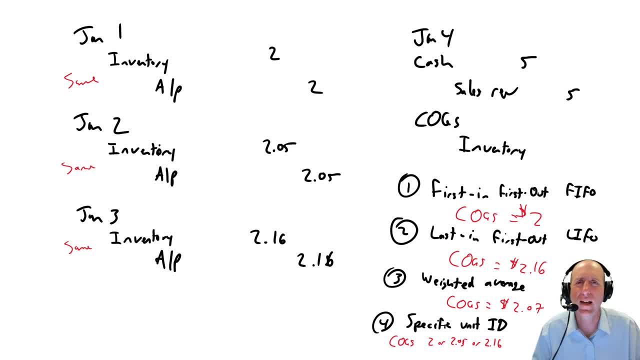 So specifically unit ID, typically for bigger ticket items like pairs of socks, you would just probably lump together. It's not worth the effort of tracking them separately. Although we could, we probably wouldn't. But with uh sort of large or unique items we might track them all separately. 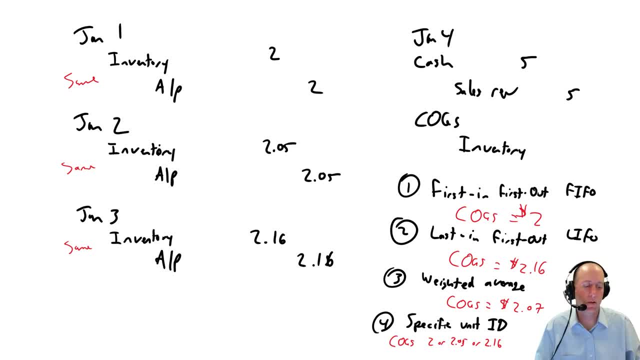 So that's a big focus of this module is just figuring out the cost of the inventory we sold. and the reality is we are allowed to use several different methods and you will be responsible, I'm sure, in your class, to understand several different methods of tracking inventory. 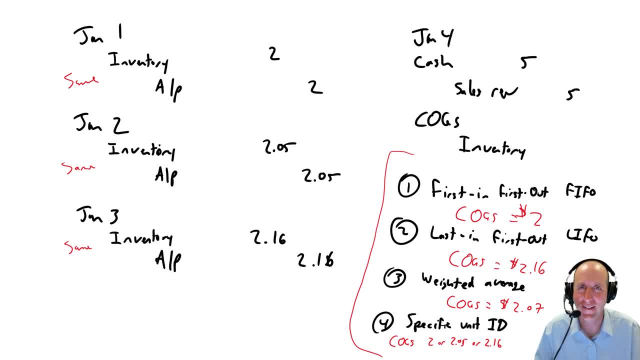 All right, I can't wait to get started. I'll see you in the next video. 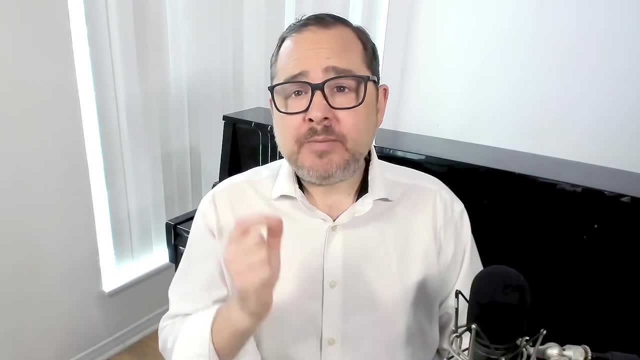 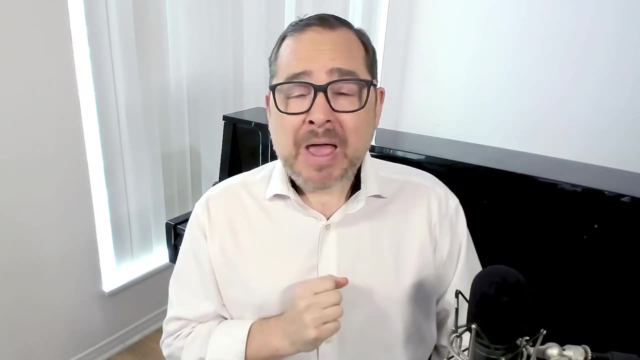 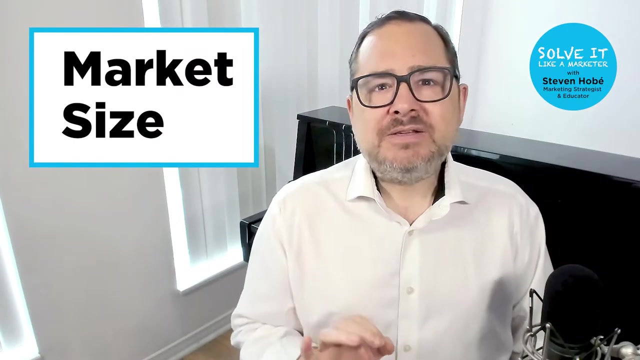 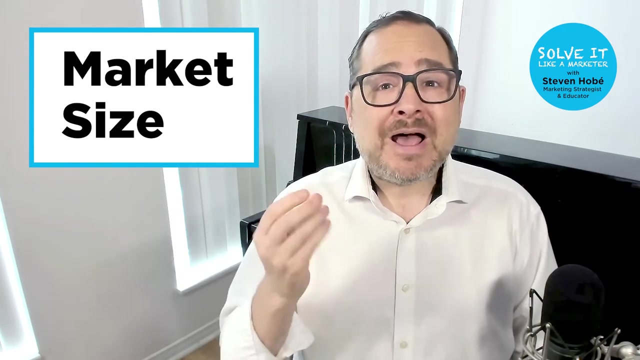 Welcome to Solve it Like a Marketer. I'm Stephen Haube. Today I'm covering calculating your market size. Now, if you like this video, please subscribe and don't go away Now. your market size is made up of the total number of potential buyers of a product or service within a given market.